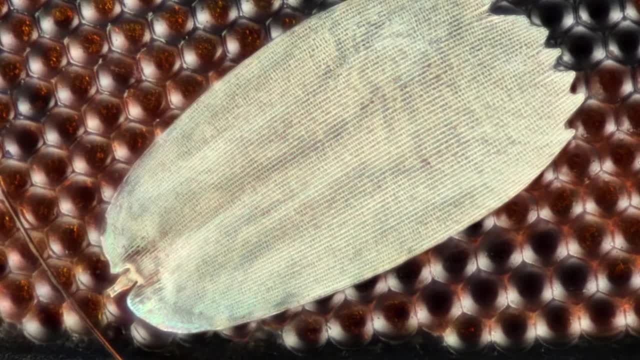 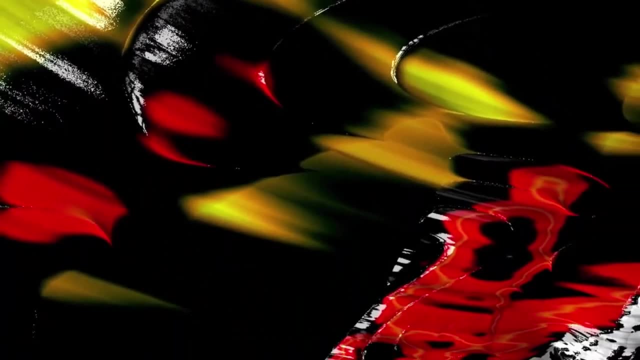 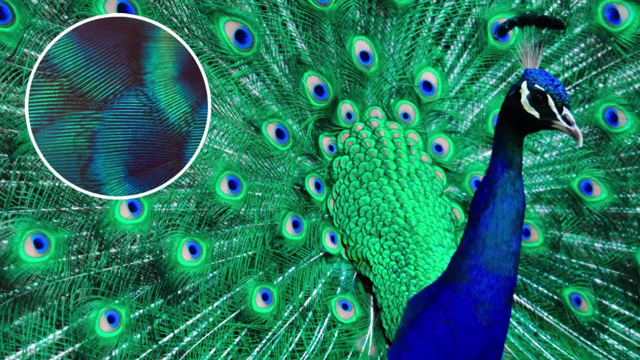 The structural colors and patterns of butterflies are different. The patterns of butterfly and moth wings come from these layers of tiny scales. As the wing moves, you will notice colors change. This is known as iridescence. This occurs when light passes through multi-layered surface, as you must have seen in peacock feathers or soap bubbles. 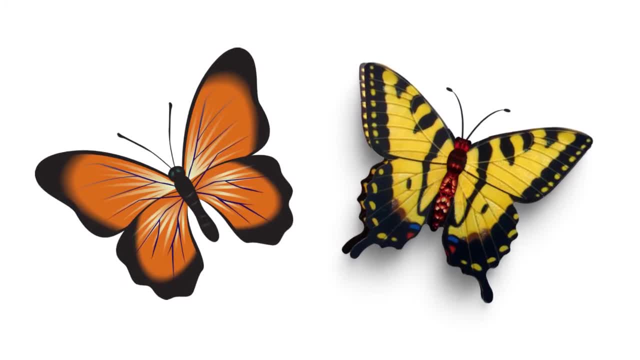 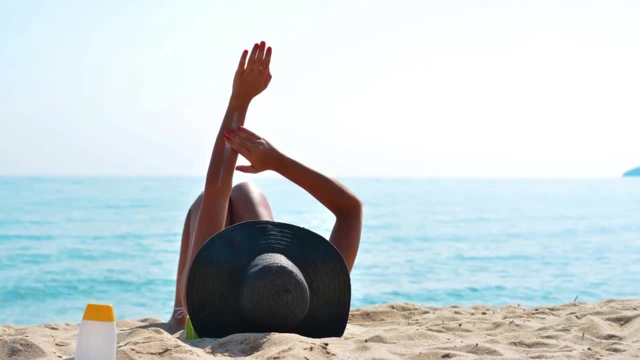 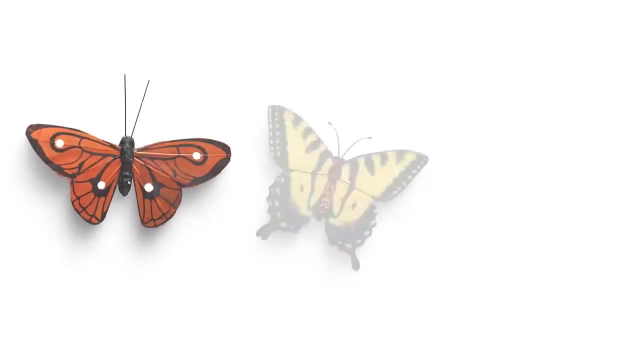 And the pigmented colors come from the chemical pigments. Most butterflies get their different shades of brown and yellow from melanin, the same pigment that makes you tan in summer. When you see blue, purple or white on a butterfly, that's a structural color, while orange, yellow and black are the colors due to pigments. 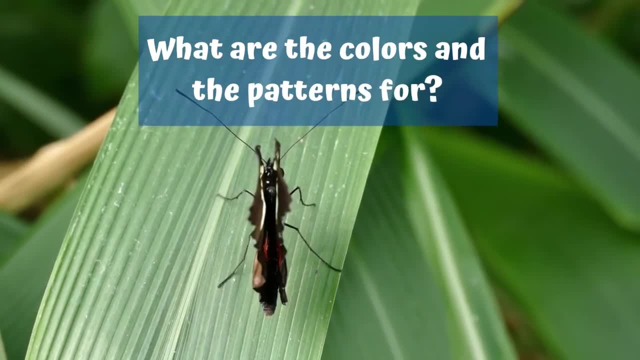 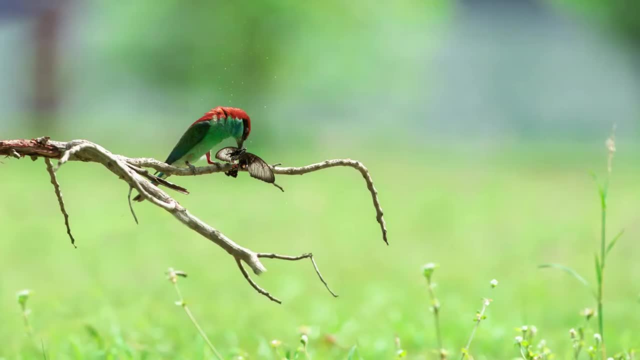 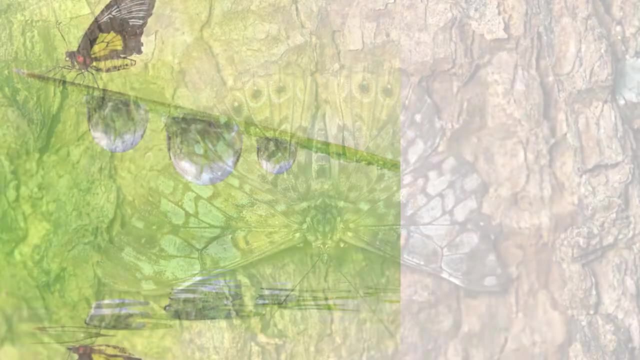 Now here comes the interesting question: What are the colors and patterns for Growing? butterflies are unable to move and is always in danger of being eaten by predators. Colors help to camouflage them from predators. A hungry bird may even think it like a drop of water, bird droppings or even a tiny snake. 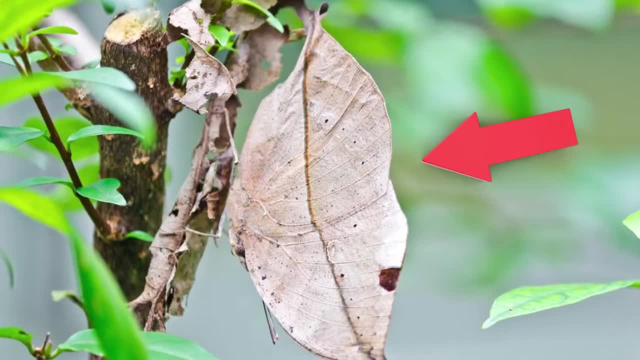 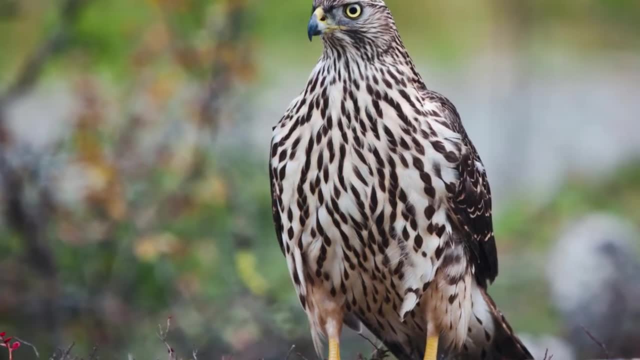 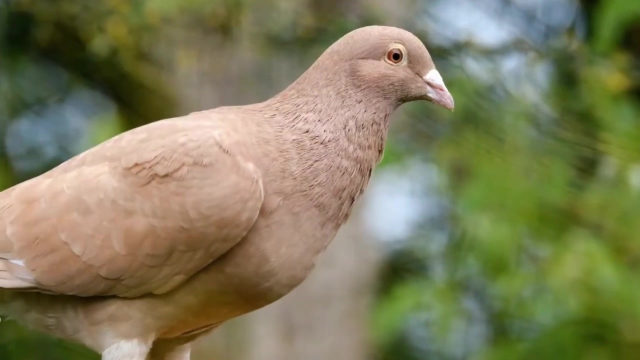 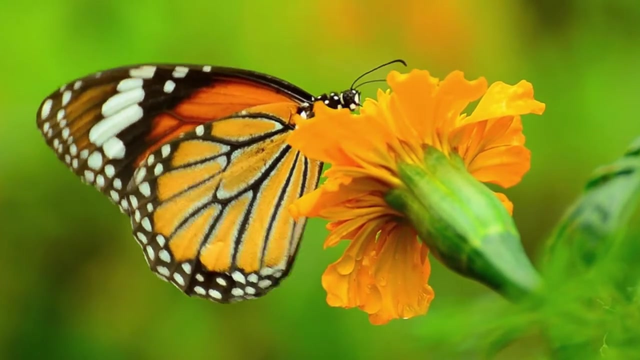 The Indian leaf butterfly is nearly impossible to spot among leaves. Some butterflies use their beautiful color to warn others of possible dangers. nearby Adult monarch butterflies have orange color and patterns which warn the predators of their toxicity or their disgusting taste. Butterflies with bright colors and patterns are advertising to predators as they are distasteful. 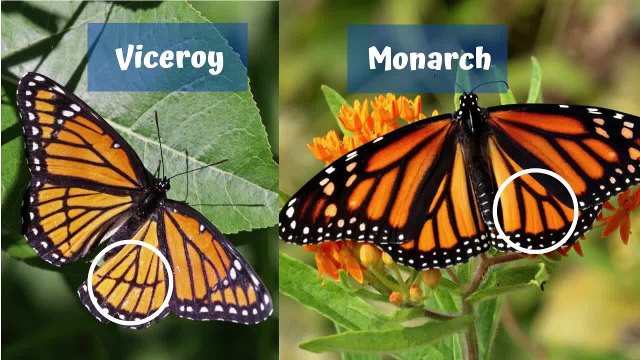 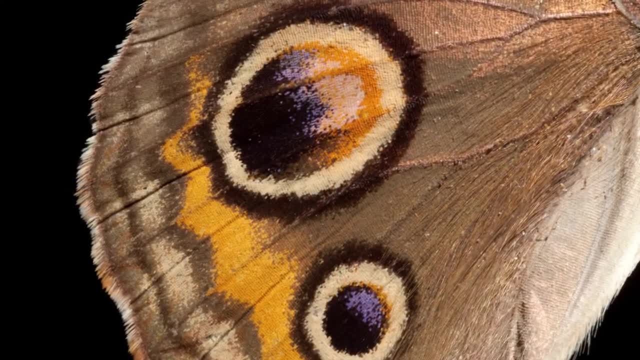 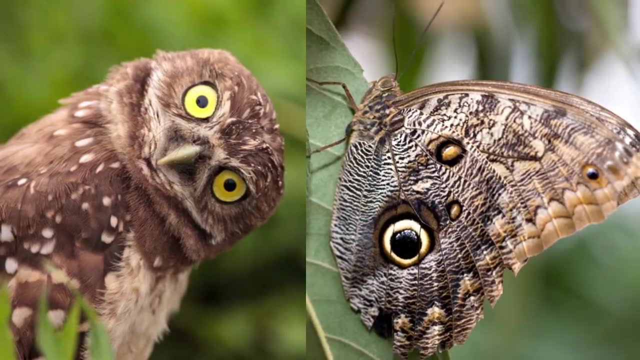 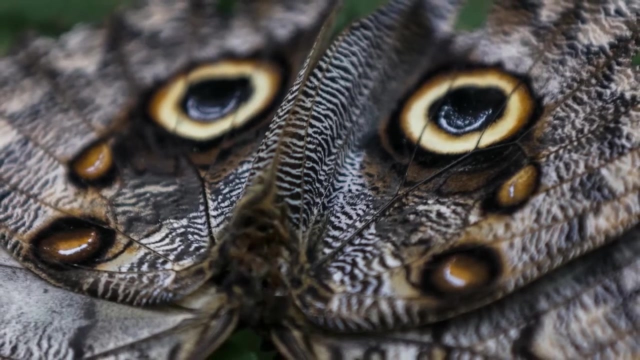 There are also butterflies like Viceroy that mimic other butterflies. that is bad tasting in hopes of fooling its predators. Others have eye spots on their wings. This tricks predators into thinking that the butterfly is actually a larger animal, such as an owl. It is thought that eye spots simply mimic the eyes of predators, making attackers think they are suddenly facing a larger and potentially dangerous animal. 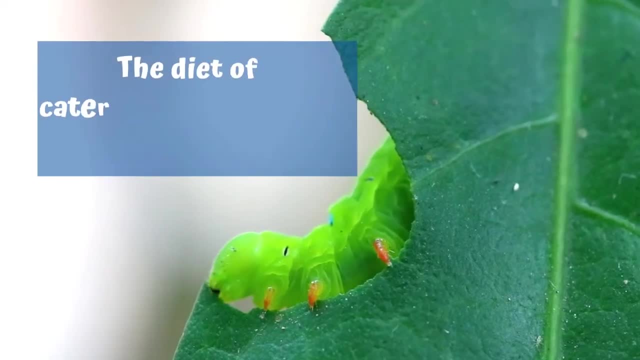 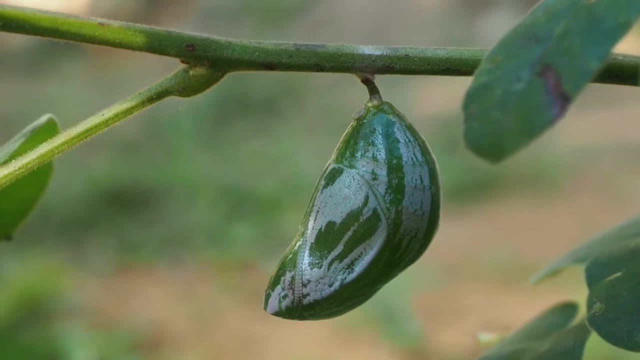 Let me tell you an interesting fact. The diet of the caterpillars affect the color of the pupa. It is because of the chemicals present in flowers, seeds and leaves influence the color of the butterfly pupas. I better fly away now before it gives me butterflies in my sleep. 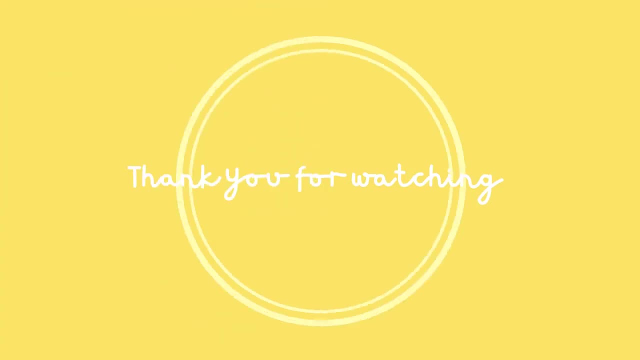 It is different seeing the butterfly pupa in the dark. I have a lot of butterflies in my belly. I may have been mistaken. I have a lot of butterflies in my stomach.